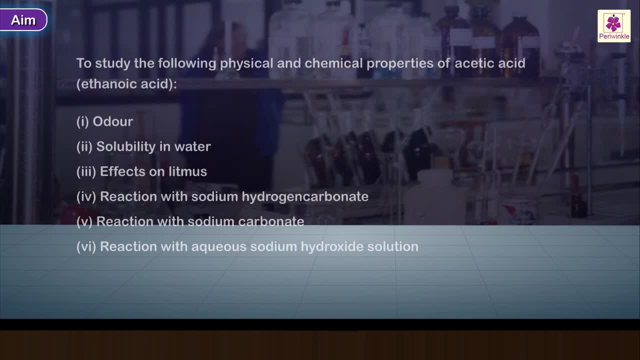 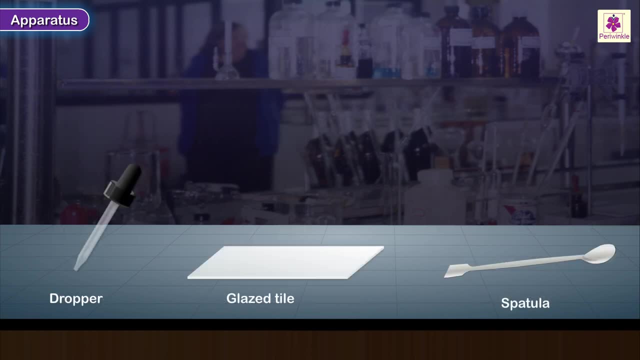 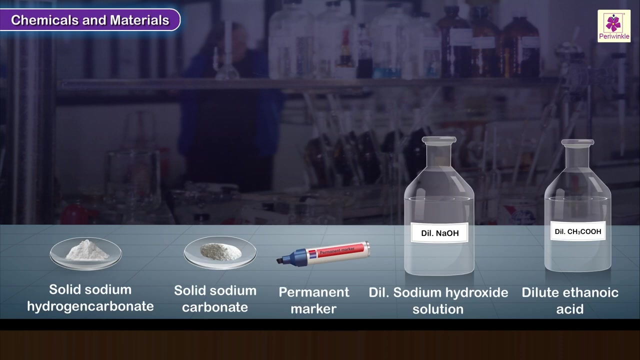 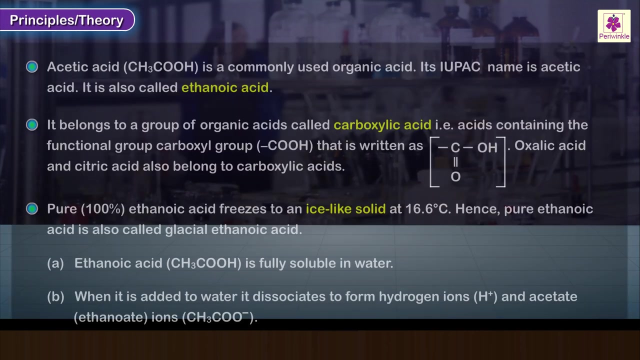 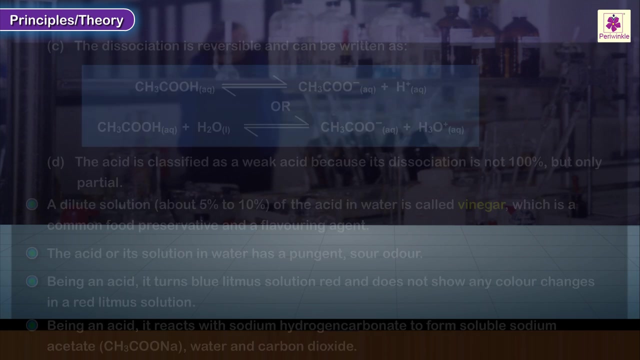 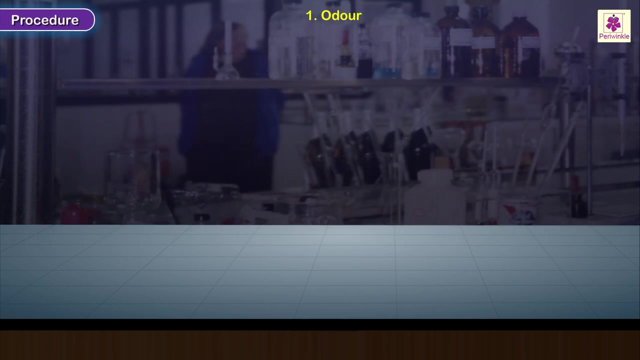 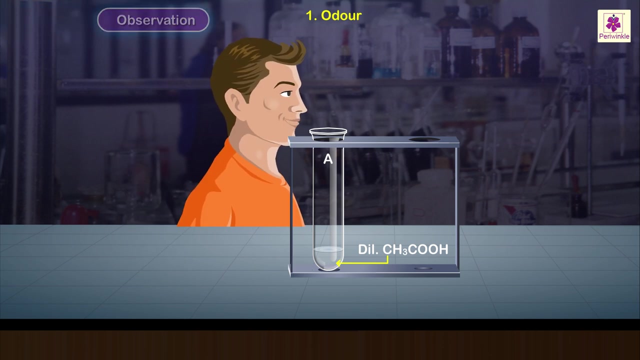 aqueous sodium hydroxide solution, apparatus, chemicals and materials, principles or theory, precautions, procedure: what order? take a testing and label it a. take about two ML of dilute ithanoic acid in the test, you a and cautiously smell it. observation and inference: the acid has applied an oil solution in a değer of 14 to a to two milliliters a. in addition to the serum treatment technologies for level, do not move the problems of mult intuitive comprehensive treatment of WWERobotics review areas. we are taking the ball Rose cette you aさん lawson will look today as possible precautions procedure 1 or d sticking a testing and label it a. take about 2 ml to dilute ethanoic acid in the test you a and cautiously smell it. observation and inferen ont anty on highacer aberra in y or serve a neighborhood. 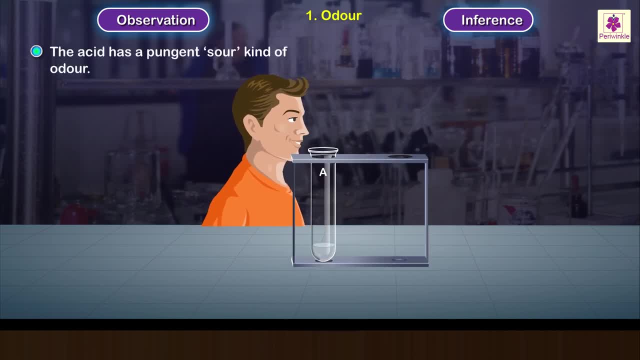 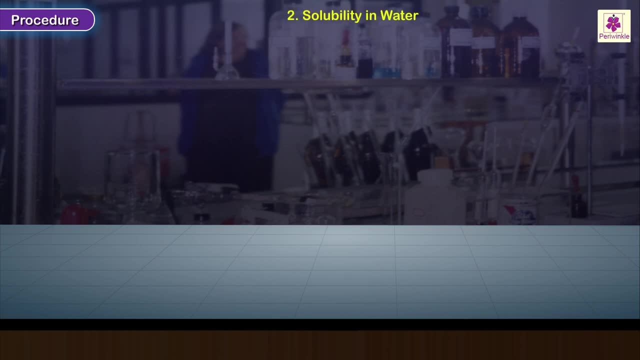 has a pungent, sour kind of odor. the odor is similar to that of vinegar. procedure 2: solubility in water. take another clean test tube and label it b. take about 2 ml of ethanoic acid in it. now add 3 milliliters of distilled water to it. 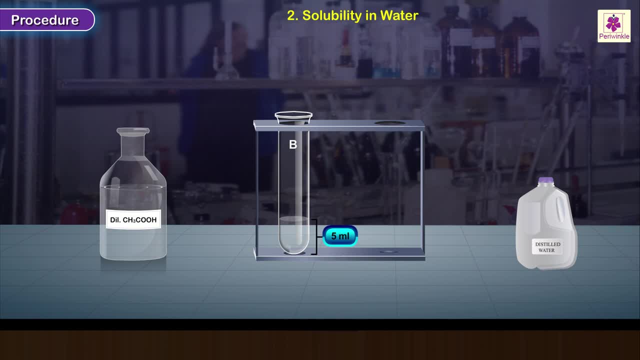 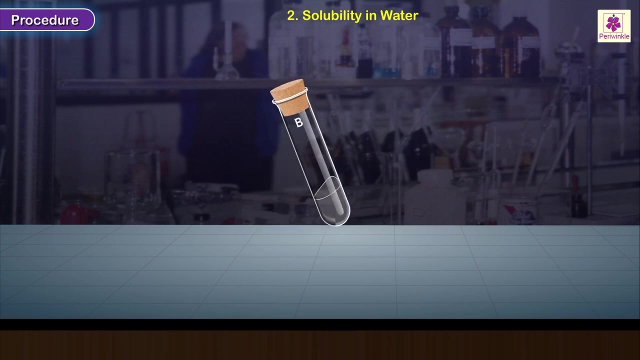 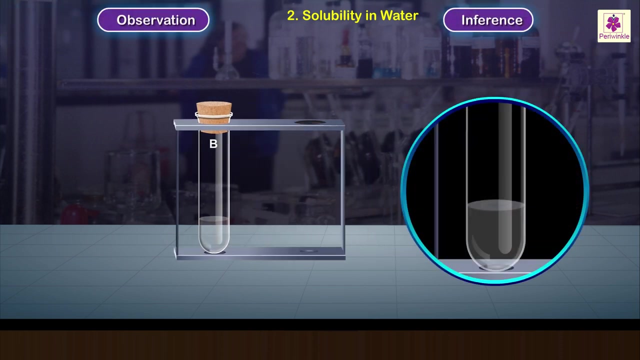 observe the mixture to find out if the two liquids have formed two separate layers. close the mouth of the test tube with a rubber stopper and agitate the contents of the test tube to mix them. well then, observe the contents. observation inference: the mixture does not show. 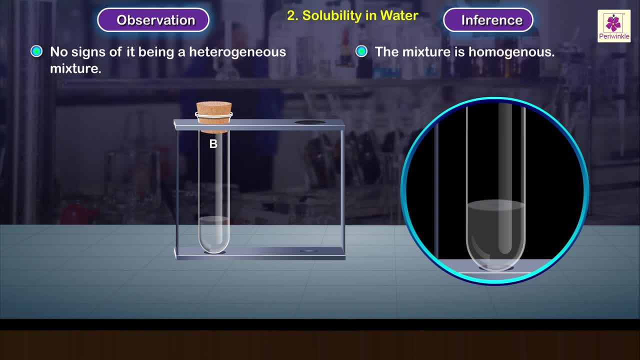 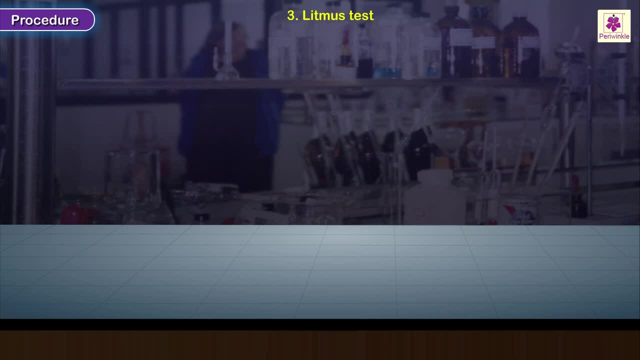 any heterogeneity nature: the mixture is homogeneous. procedure 3 litmus test. take two test tubes and label them as c and d. take about two ml of dilute ethanoic acid in each. add a drop of blue litmus solution to the contents of the test tube C and a drop of red litmus solution to the test tube D. Gently shake. 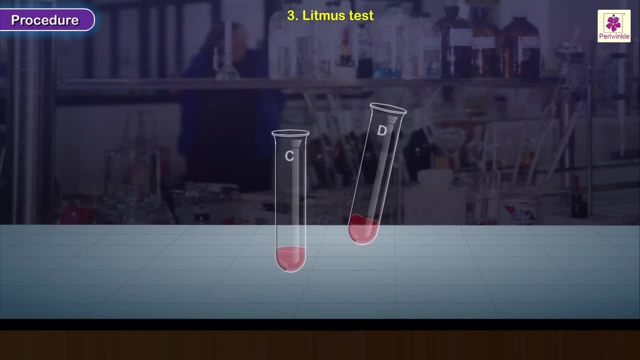 the test tube, or take a blue and a red litmus paper strip and place them on the white surface of a smooth glazed tile. Then, using a dropper, drop one to two drops of ethanoic acid on each litmus paper. Observations: 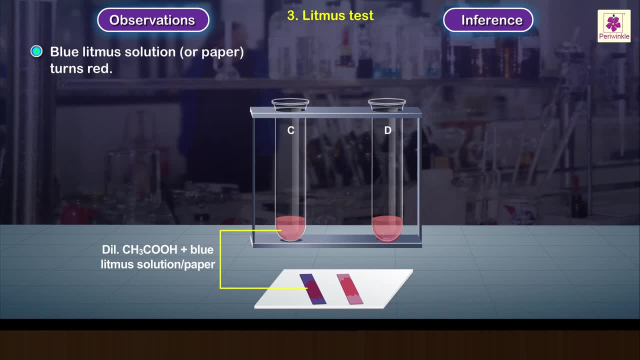 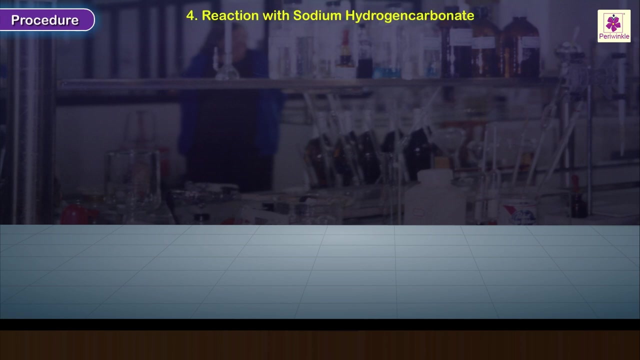 Inference: Blue litmus solution or paper turns red and red litmus solution, or paper turns yellow. The solution is acidic in nature. Procedure 4. Reaction with sodium hydrogen carbonate. Take one to two grams of solid sodium hydrogen carbonate in a test tube that has a side tube. Add about five ml of dilute ethanoic acid to. 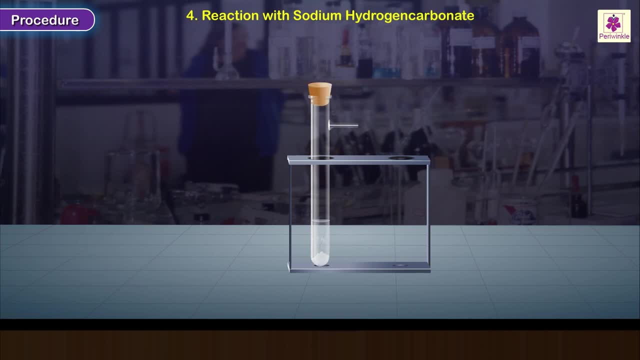 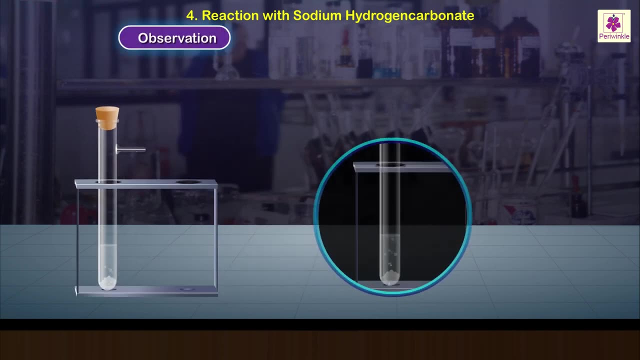 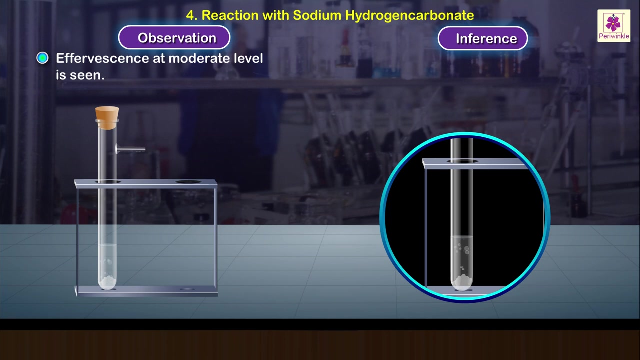 the test tube, Close its mouth with a rubber stopper and observe its contents. Observation Inference: Effervescence at moderate level is seen. At least one of the products is a gas when ethanoic acid and sodium hydrogen carbonate react with each other. 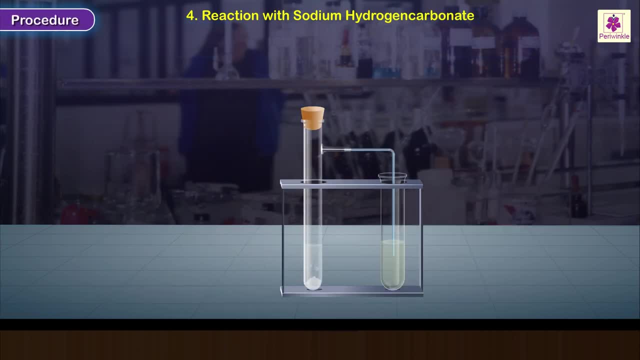 Procedure 5.. At least one of the products is a gas. when ethanoic acid and sodium hydrogen carbonate react with each other. After about a minute, take the mixed solution of the two ingredients mixed with one and add the scream organic acid with one of them. 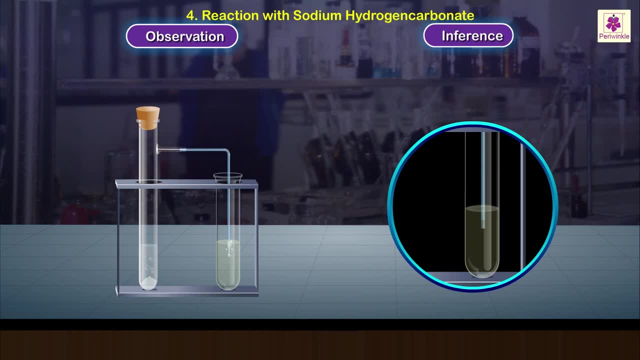 At this point. take this liquid with a small amount of de�ate and add it to your glass. When this liquid is added, add the deaky liquid with a little bit to the solution. If you see that the solution is not enough, make the solution of the solution for this. 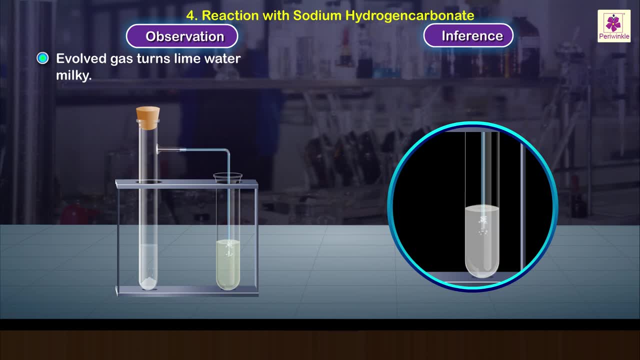 as the solution is already very rich in rocket sense. Not enough is enough. Add the desired amount of denenol to the solution as well as this one. As the solution is still very thin, add one to two grams of denenol to the solution. 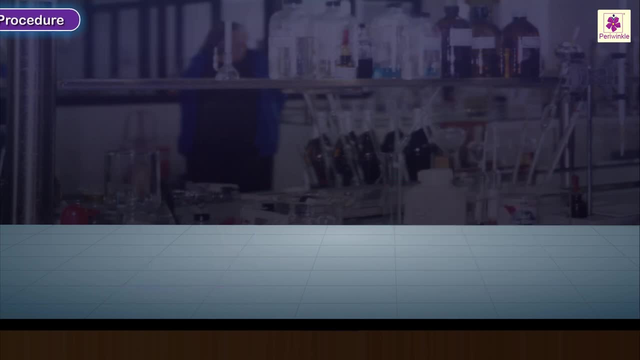 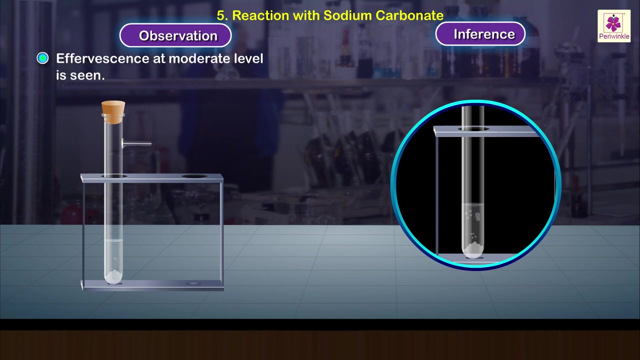 The solution is ready. Now enter the solution of the solution In the same way. add the solution of the solution to the solution. five: reaction with sodium carbonate. repeat earlier procedure using sodium carbonate instead of sodium hydrogen carbonate. observation inference: effervescence at moderate level is seen.